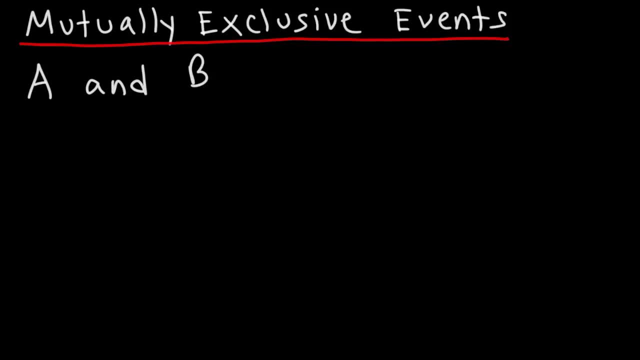 do not share any outcomes. Now what we're going to do is illustrate this with an example. Let's say we're rolling a six-sided die with a sample space of one to six. Now let's say that event A represents the outcomes one, two and three. Now let's say that event B 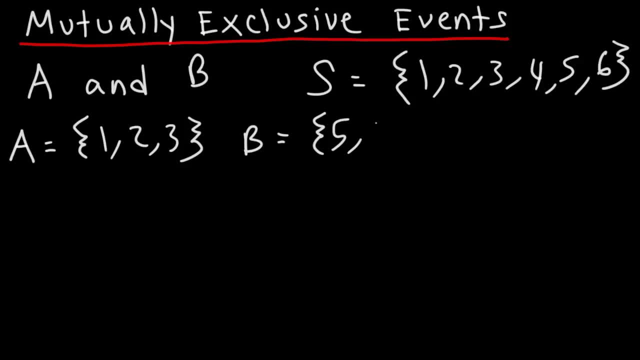 has A, two and three. So what does that mean? Now let's say that event B has A, two and three, has the outcomes five and six, whereas event C, we're gonna say, has the outcomes three, four and five. 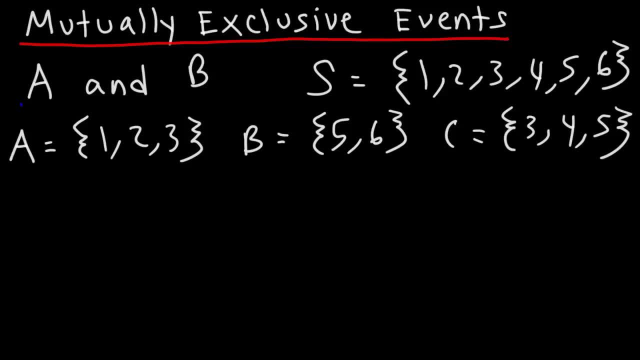 Now here's the question: A and B are they mutually exclusive events? What would you say? What is the sample space of A and B? What is the intersection of these two events? Notice that they do not share any outcomes, So there's no intersection. 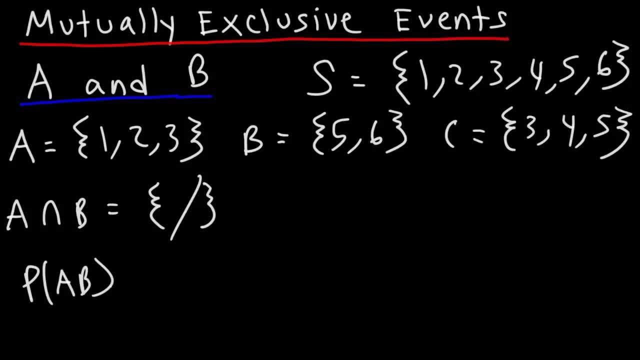 Therefore, the probability of A and B occurring together is zero. this cannot happen. Let me write this as A and B, because you might think it's A then B, So make sure you understand this. The probability of two mutually exclusive events. 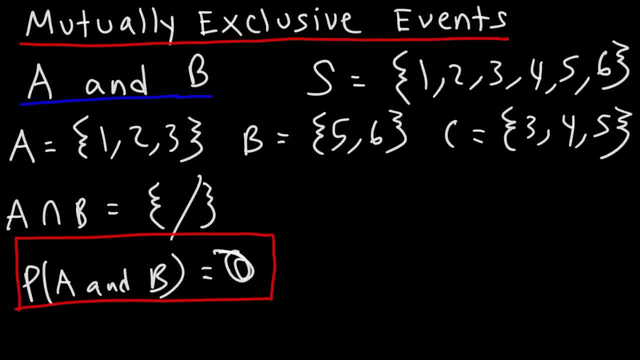 occurring is always gonna be zero. Now what about events A and C? Are they mutually exclusive? Notice that A and C, they share the outcome three. So the intersection of these two events is three. So the probability of getting A and C. 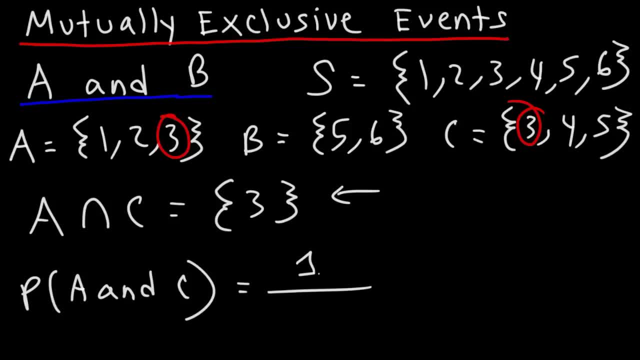 is going to be this one outcome over three. So the probability of getting A and C is going to be this one outcome over the six possible outcomes. So, because the probability of getting A and C is not zero, A and C are not mutually exclusive events. 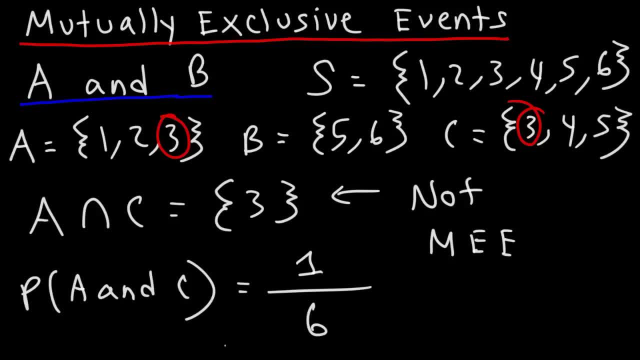 However, A and B, they are mutually exclusive events. Now, what about events B and C? Are they mutually exclusive? B and C, they share the outcome five. So that's the intersection of these two events. So that's the probability of getting B and C. 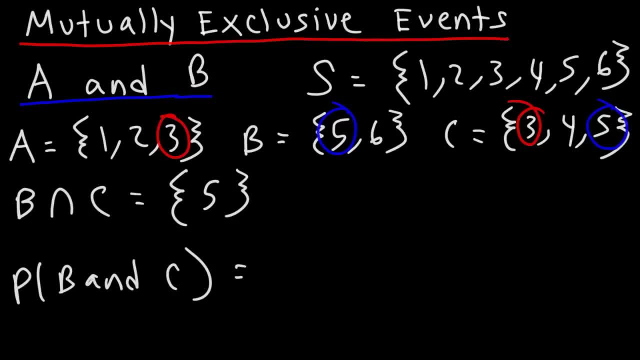 is going to be the same. it's one over six. So because it does not equal zero, we can say that B and C are not mutually exclusive events. So that's how you can use B and C to verify B and C. 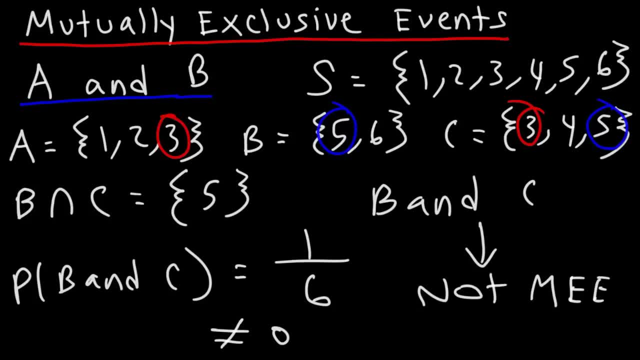 Let's see B. You can tell if two events are mutually exclusive or not. You need to find the probability of getting those two events. If it's zero, they are mutually exclusive. If it's anything but zero, they are not mutually exclusive. 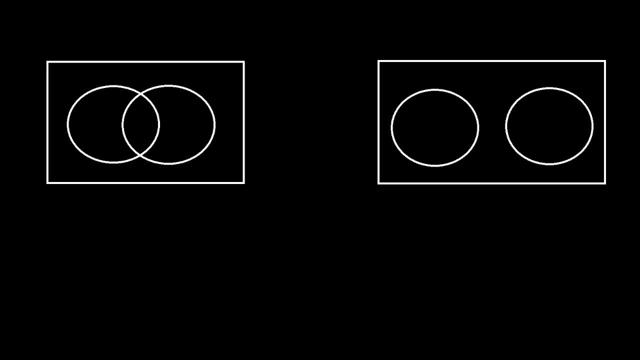 Now let's illustrate the concept of mutually exclusive events using Venn diagrams. So let's say this is event A and on the right, event B. So which Venn diagram would you say represents mutually exclusive events? Is it the one on the left or is it the one on the right? 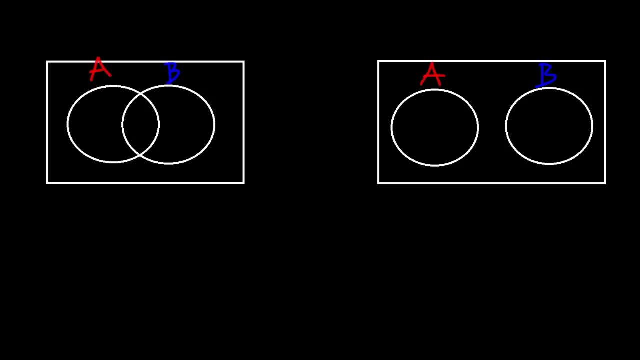 Now we know that mutually exclusive events do not share any outcomes. So the one on the right are mutually exclusive events. The one on the left are mutually exclusive events. The one on the left are not mutually exclusive events, because they do share something in common. 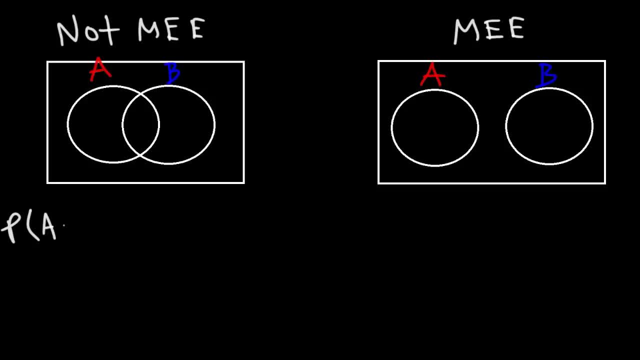 Now, how can we calculate the probability of getting event A or event B for something that's not mutually exclusive? This is the same as A in union with B, and it's equal to the probability of getting event A plus the probability of getting event B. 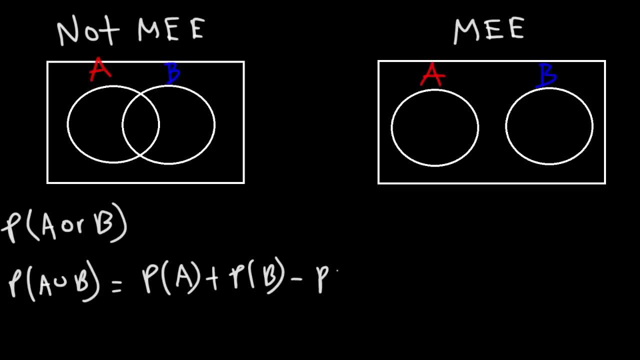 So the probability of getting event B minus the probability of getting both A and B, That is the intersection of A and B. So this equation works for events that are not mutually exclusive. Now, that doesn't mean it doesn't work for events that are mutually exclusive, because 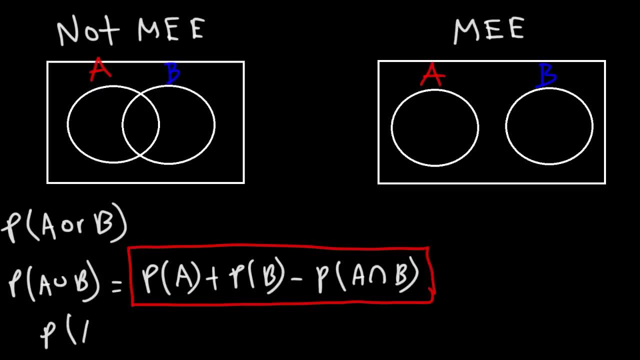 it does Keep in mind for a mutually exclusive event or events, rather, The intersection of A and B will be zero. So therefore, the probability of getting A or B for two mutually exclusive events is simply PA plus PB. If you use this equation, this will be zero and it will still work. 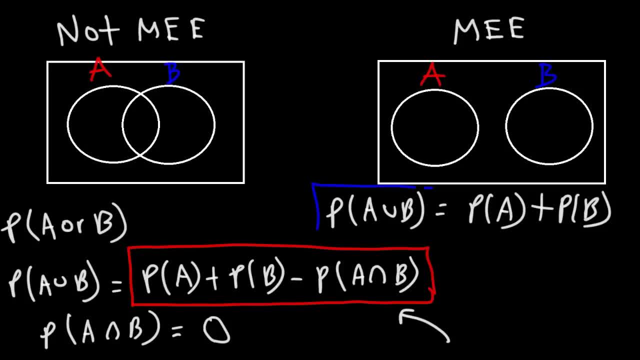 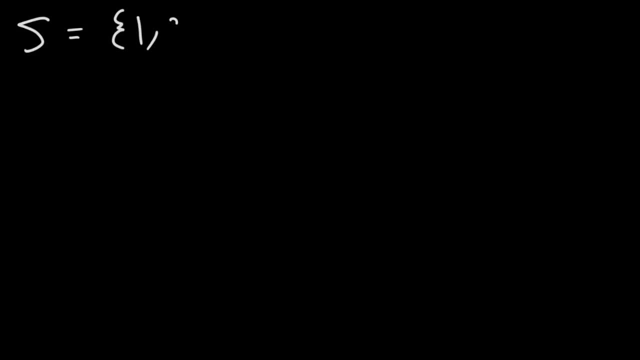 It simply simplifies to the equation that we have on the right if you have two mutually exclusive events. Now let's work on some example. Let's work on some example problems. Let's use our favorite six sided die with a sample space of the natural numbers from: 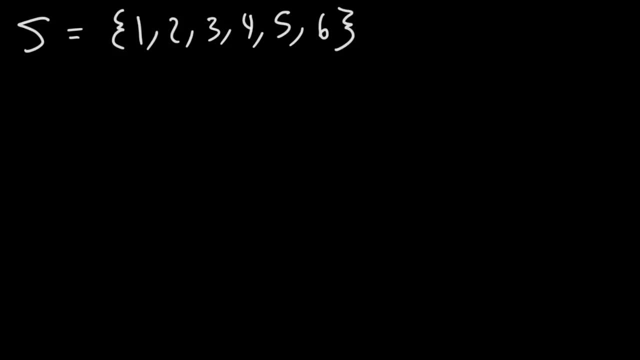 one to six. Now let's say that event A represent the outcomes one, two, three and four. Let's say that event B represent the outcomes three, four and five. What is the probability of getting A or B? What is the probability of getting A or B? 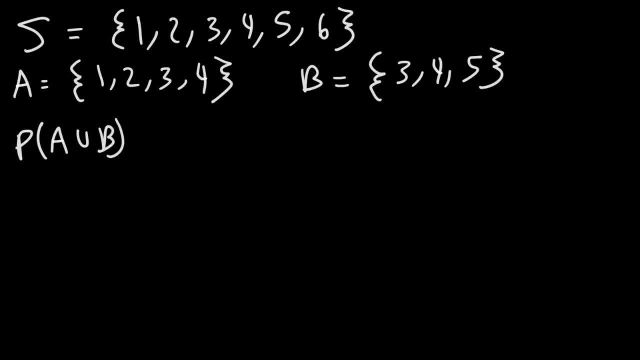 By the way, are these events mutually exclusive? We could see that they're not, because they share the outcomes three and four. So let's represent this with an event diagram. So, because they're not mutually exclusive, we need to draw this way. 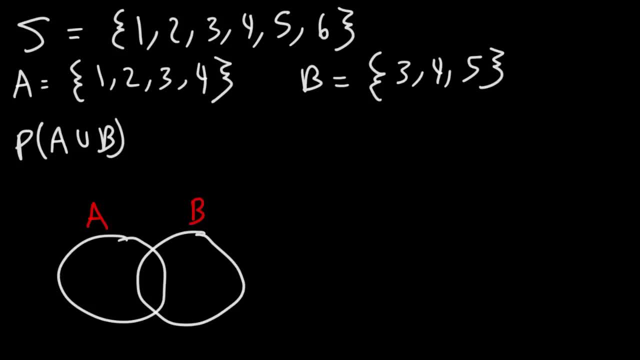 This is going to be A and this is going to be B. Now, A and B have the numbers three and four in common, So we're going to put that in the middle. A also has one and two. B has five. The probability. well, let's write the formula for this first. 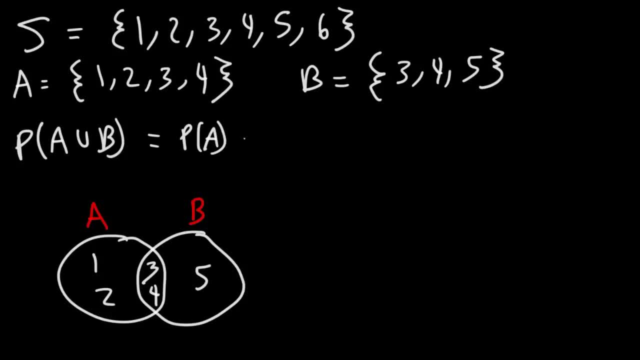 So P of A or B is going to be P of A plus P of B, minus the probability of getting both. Now what is the probability of getting event A? There's four outcomes that relate to event A out of a total of six potential outcomes, so it's going to be four over six. 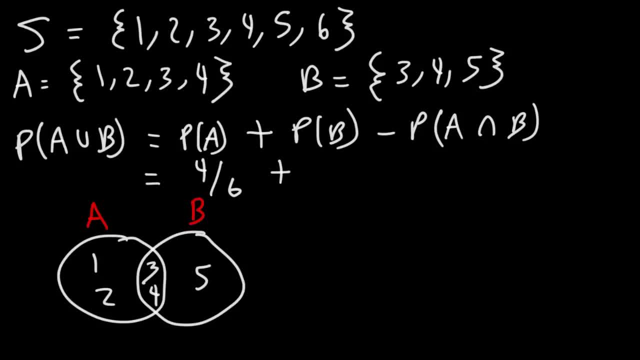 Now, what about the probability of getting event B? Notice that there's three outcomes that relate to it, so it's going to be three out of six If we were to ignore this part of the equation. notice that if we add these numbers, this: 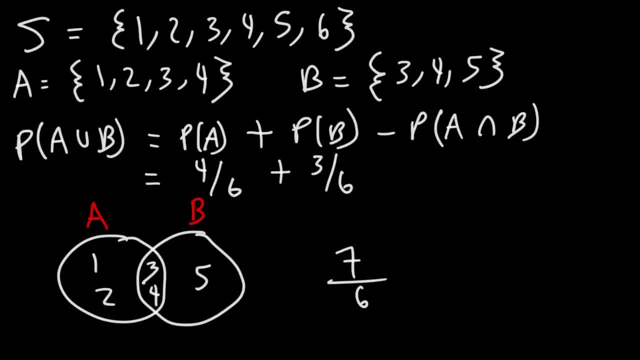 would be seven out of six, and this is not possible. The probability of any event occurring cannot be more than one. It can't be greater than 100%, so that's why this part of the equation has to be there. We have to deduct the events that occur in common, otherwise we'll be counting three. 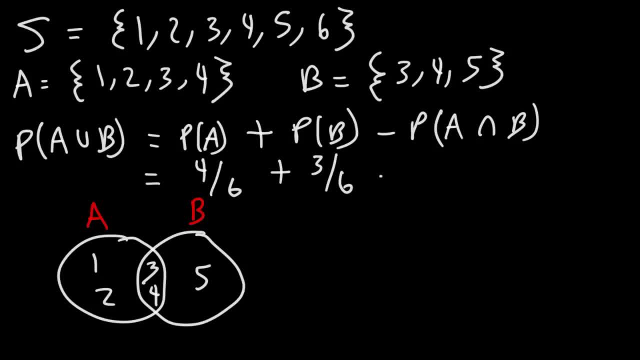 and four, twice So the probability of A and B occurring. This represents two outcomes out of a total of six, so it's two over six. So if we add four and three, which is seven, and then subtract that by two, we get five. 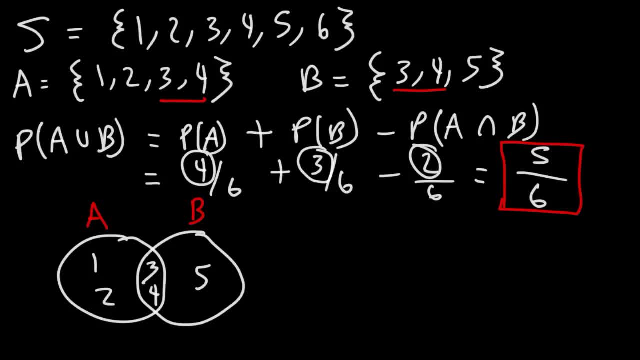 over six. So that's the probability of event A or B occurring. Now let's see if this answer makes sense. So what is the union of A and B? What is the sample space for that? A has the numbers one to four. 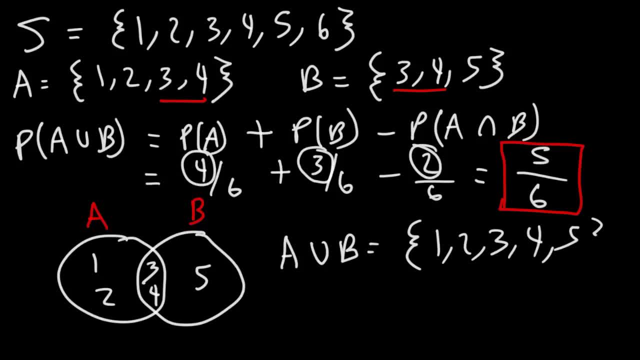 B has the numbers three, four and an additional number five. So the sample space of A or B is the numbers one through five. So to calculate the probability of A in union with B using this, we have five favorable outcomes out of a total of six. 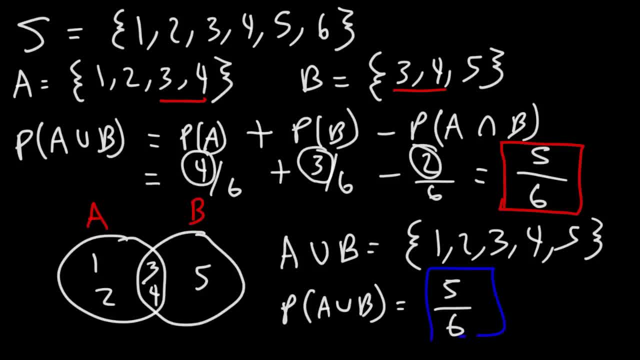 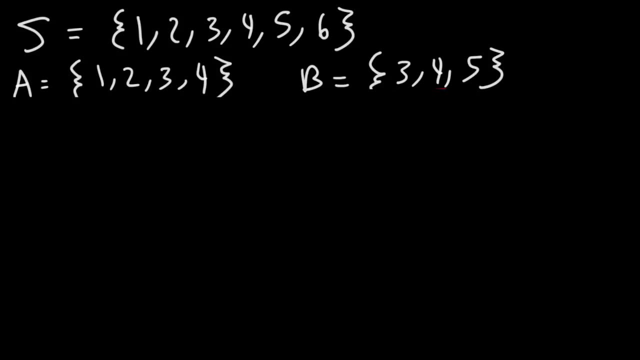 So we could see why the probability is going to be five over six. So hopefully this equation makes sense. Now you see why it works the way it does. Now let's add a new event in this problem. We're going to add event C, and C is going to have the outcome six. 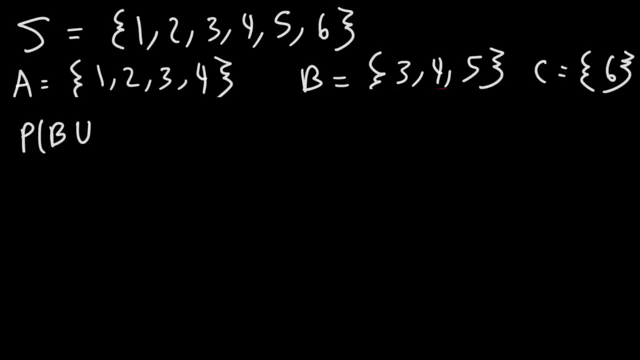 What is the probability of getting B or C? So let's write out the formula. This is going to be the probability of B or C. So let's write out the formula. This is going to be the probability of getting B plus the probability of getting C minus. 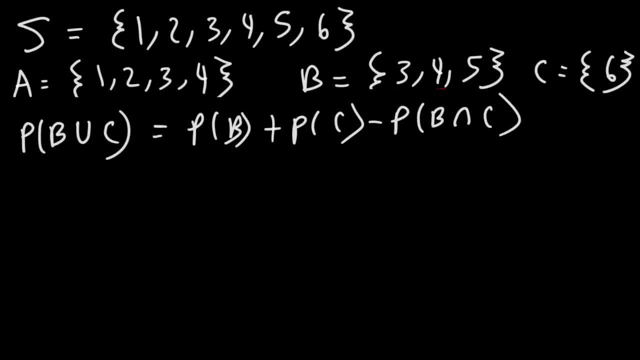 the probability of getting B and C. Are these events mutually exclusive? What would you say? Notice that B and C do not share any outcomes. So this is a mutually exclusive event: B and C. So if we were to draw an event diagram,